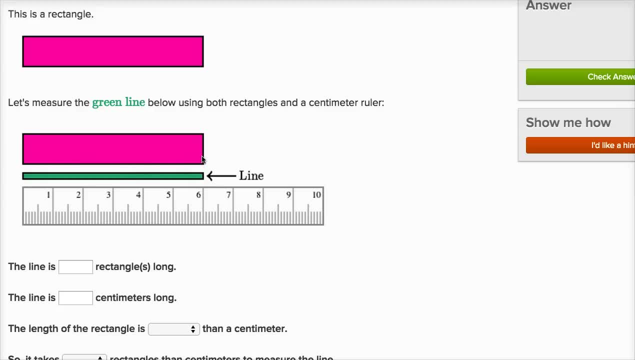 And you immediately see the green line is equal to one rectangle long, but if we measure it in centimeters, it's equal to six centimeters long. So we could say: the line is one rectangle long, but it's six centimeters long. 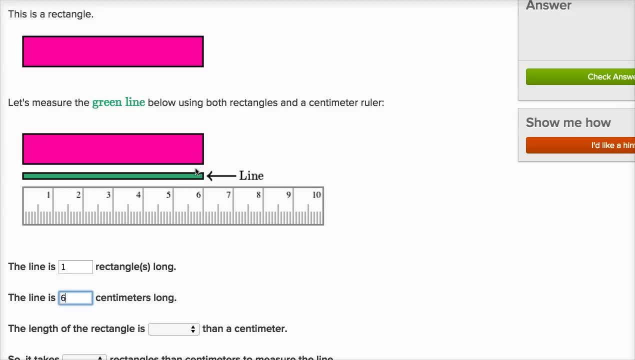 And that makes sense, because the rectangle is much more than a centimeter. It's actually, the length of a rectangle is six centimeters, So the length of a rectangle is longer than a centimeter. You see that This is the length of the rectangle. 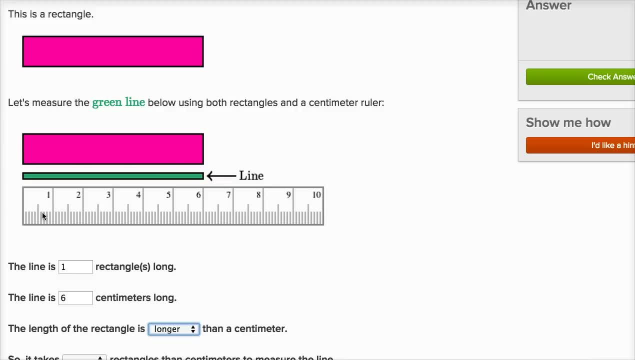 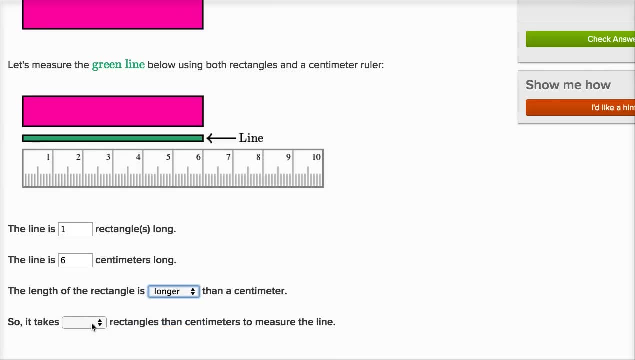 It's the same as a line. while a centimeter is this length, The rectangle's actually six centimeters long, So it takes blank rectangles than centimeters to measure the line. Well, since the rectangle is longer, it takes fewer rectangles than centimeters. 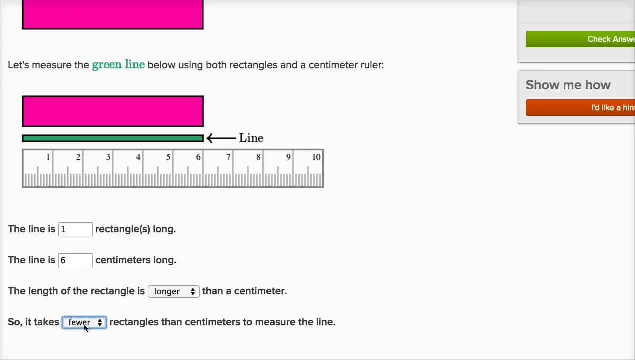 to measure the line. So it's fewer rectangles than centimeters and you see that Fewer rectangles One is fewer than six. It only took one rectangle to measure the line because the rectangle's so long and it took six centimeters to measure the line. 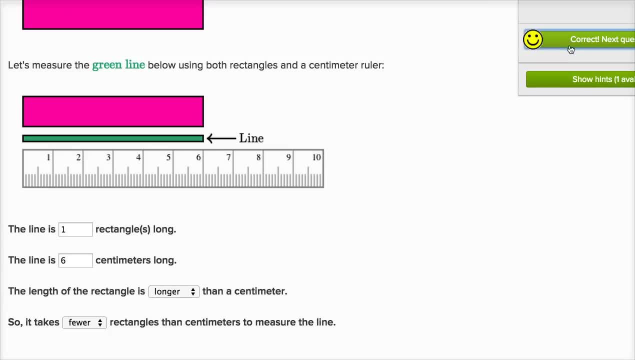 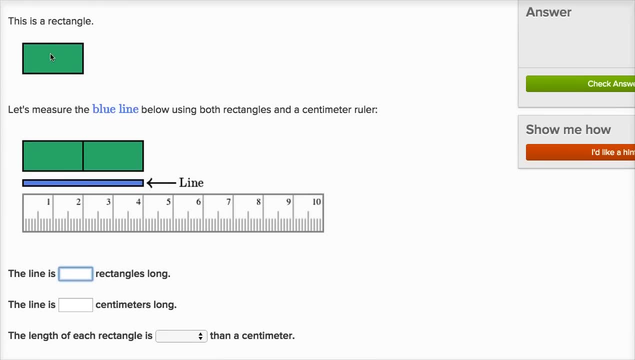 So it took fewer rectangles than centimeters to measure the line. Let's keep going. All right, So we have: this is a rectangle. Yes, that is a rectangle. Let's measure the blue line below using both a rectangle and a centimeter ruler. 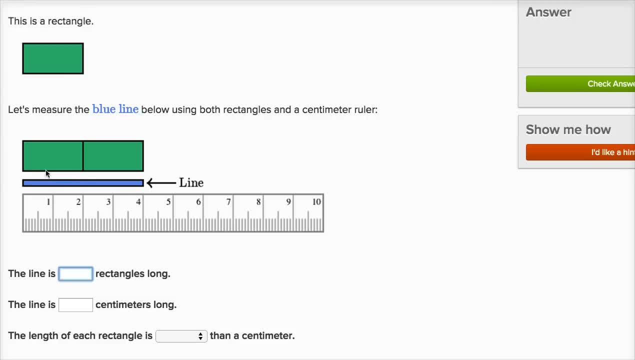 So it's a similar idea. So when we look at this blue line, the line is now two of these green rectangles long, So it is two rectangles long. Now, in terms of centimeters, it is four, four centimeters long. 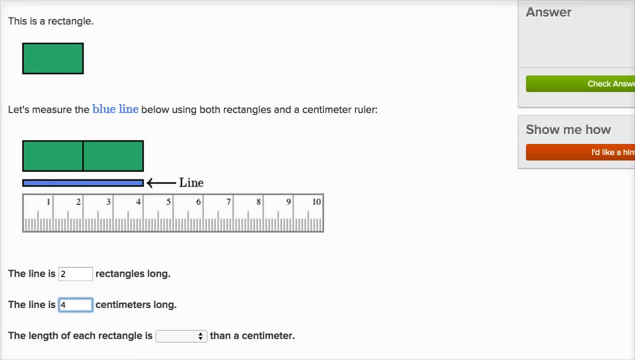 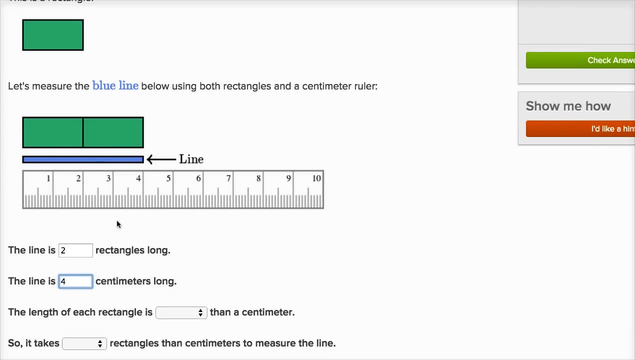 Four centimeters long. The length of each rectangle is blank than a centimeter. Well, each rectangle is more than a centimeter, It's longer. You see, each rectangle's actually two centimeters, So it's longer than a centimeter. 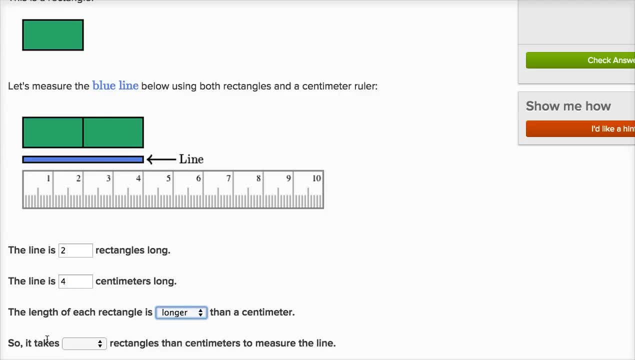 It takes blank rectangles than centimeters to measure the line. Well, since each rectangle is longer, it's going to take fewer rectangles to measure the line, So we'll select fewer right over there, And you see that over here It only took two rectangles to measure the line.